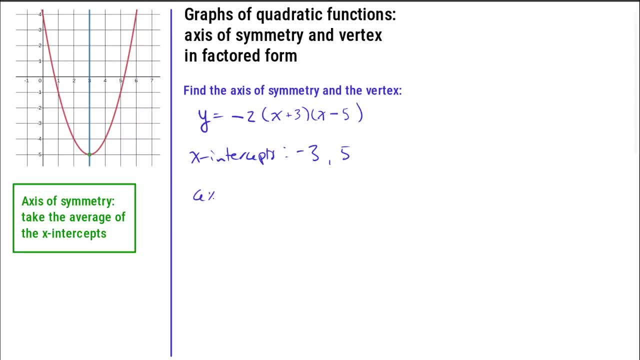 And then we just take the average, the midpoint, Because this axis of symmetry it's going to be halfway between two points at the same height. Negative 3 and 5 are at the same height, So the axis of symmetry will pass through the midpoint between them. 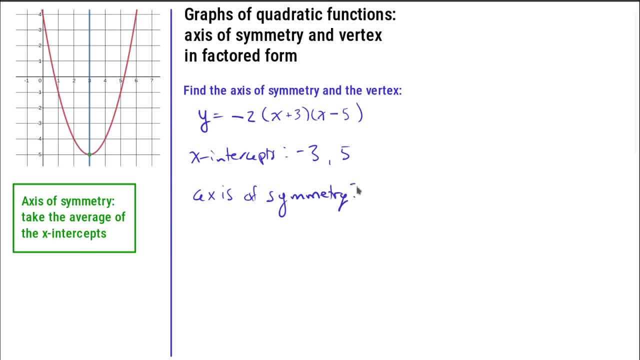 So our trick is to take the average, So it's the average of negative 3 and 5.. And the way averages work, you add the two numbers up and divide by 2.. So negative 3 plus 5, that's 2, and then 2 in the denominator. 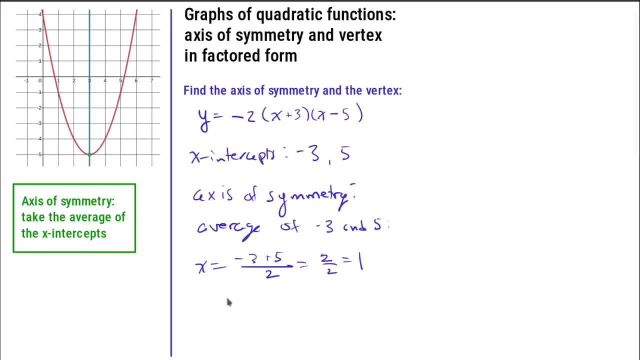 2 divided by 2 is 1.. So our axis of symmetry is: x equals 1.. So you can always, if you have both x-intercepts, find the midpoint or the average and that'll give you the axis of symmetry. 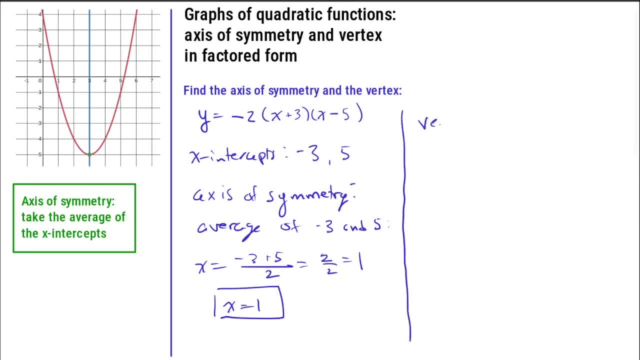 And then to find the vertex, just like we do when we're looking for the vertex. in standard form we plug in the x-coordinate to find the y-coordinate. So we know that x equals 2 is the x-coordinate of the vertex, because the vertex is on the axis symmetry. 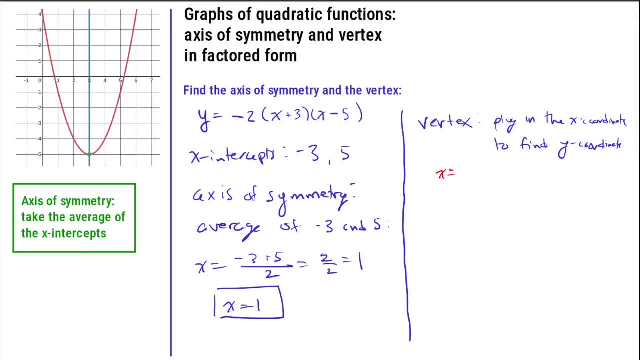 And sorry, that's not an x equals 2, that should be x equals 1.. Sorry about that. x equals 1.. And then we go back to our original equation: y equals negative 2, x plus 3.. x. 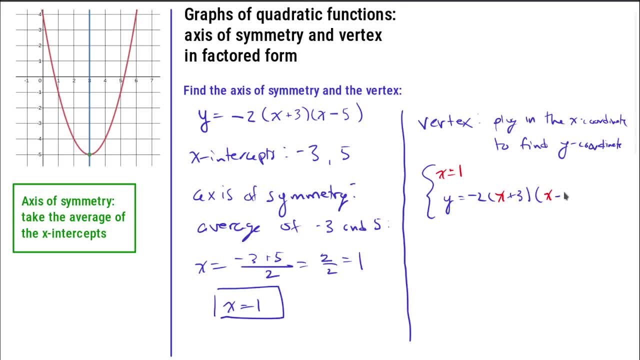 Minus 5.. And we substitute 1 for x and solve for y. So y equals negative 2, 1 plus 3, times 1 minus 5.. And we simplify using order of operations: Negative 2, 1 plus 3 is 4.. 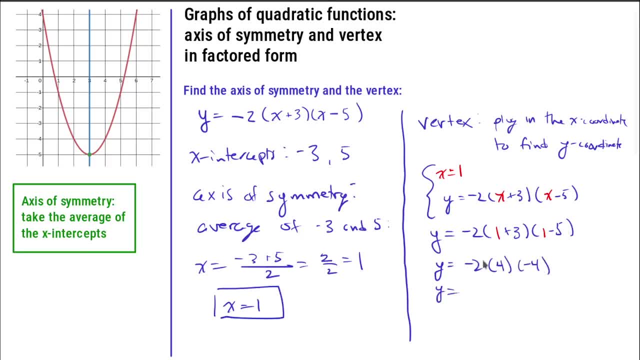 1 minus 5 is negative 4.. Negative 8 times negative. 4 is the negatives are going to cancel. We are going to end up with positive 32.. Okay, so the x-coordinate was 1. And now we've just shown that the y-coordinate is 32..